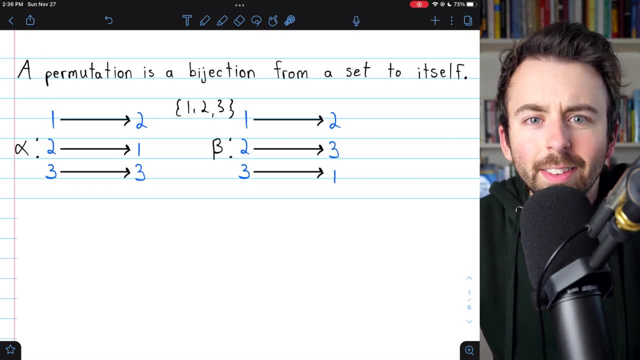 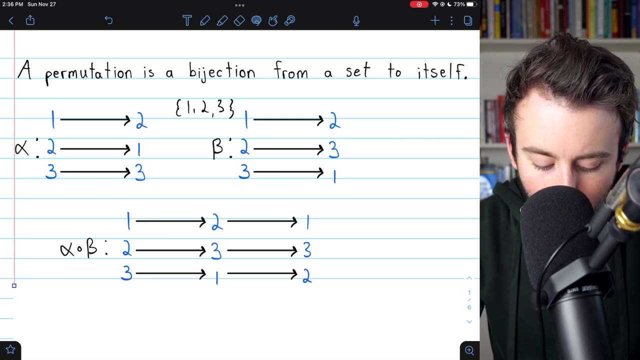 We're thinking about how groups are constructed with permutations, so what would the operation be between permutations? Well, again, a permutation is just a special type of function, so the operation is function composition, and it works quite simply. If we want to compose the permutation alpha with the permutation beta, we would write it like this, alpha of beta. Just remember how the notation works. This means that the permutation beta is applied first, and then alpha is applied. So we start with 1, 2, 3, and first we apply beta. That sends 1 to 2, 2 to 3, and 3 to 1. And then we apply alpha, which takes 2 and sends it to 1. It takes 3 and sends it to 3, and it takes 1 and sends it to 2. So the net effect of composing alpha with beta 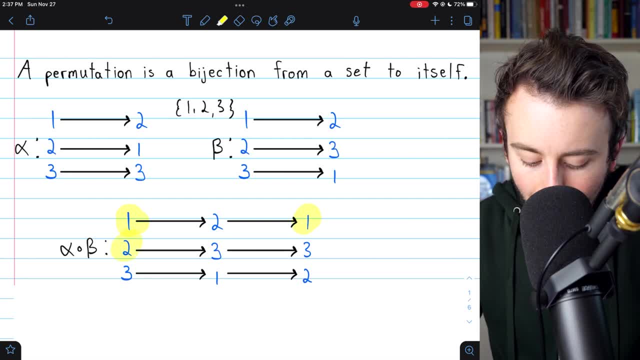 was to send 1 to 1, 2 to 3, and 3 to 2. It gave us another permutation. So we've got 2, 2, 3, and 3 to 2. And then we apply alpha, which takes 2 and sends it to 1, 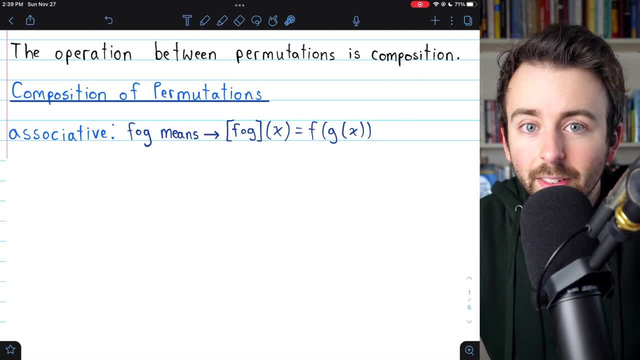 We've got this idea of permutations, bijections from sets to themselves, 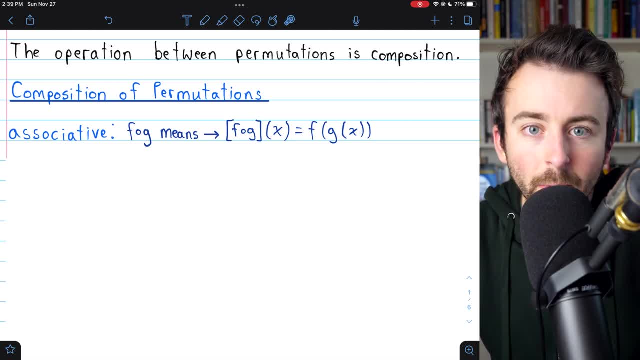 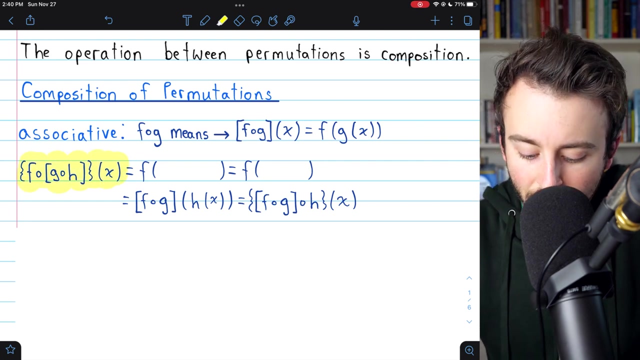 and we've got this operation between them, composition. Now, let's discuss some properties that this operation has. Firstly, it is associative. This is because function composition is associative. So the composition of permutations is associative as a result. To quickly prove it, let's just recall what function composition is. Its notation is this, f of g of some input x. And what it means is evaluate the function f at the function g at x. So f of g of x is f of g of x. To prove this operation is associative, we need to show that f composed with g of h of x is equal to f of g composed with h of x. And this is done through repeated applications of the data. 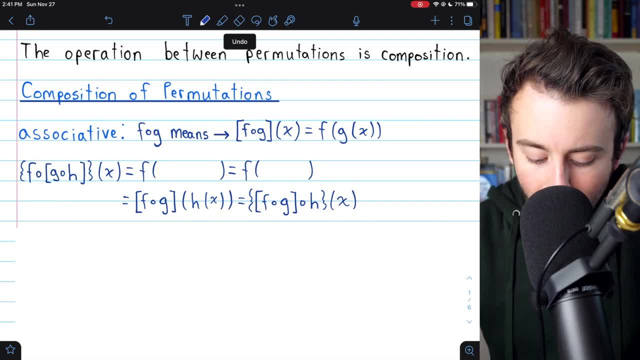 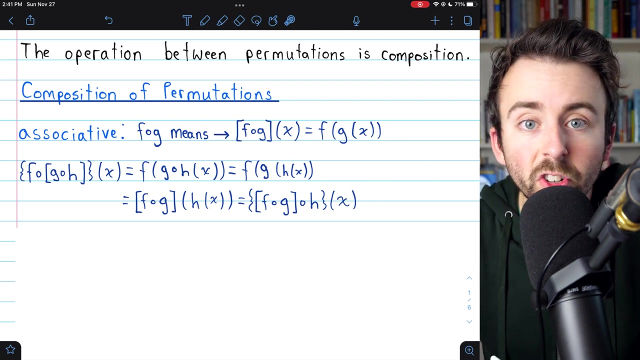 F composed with g of h is by definition f of g composed with h. But then f of g composed with h is by definition f of g of h. But then f of g evaluated at h of x is just f composed with g evaluated at h of x, which by definition is f composed with g of x. 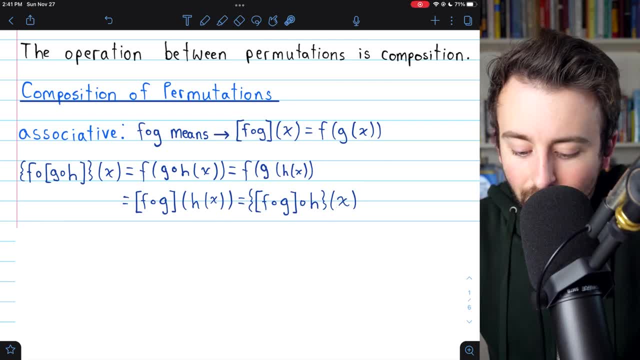 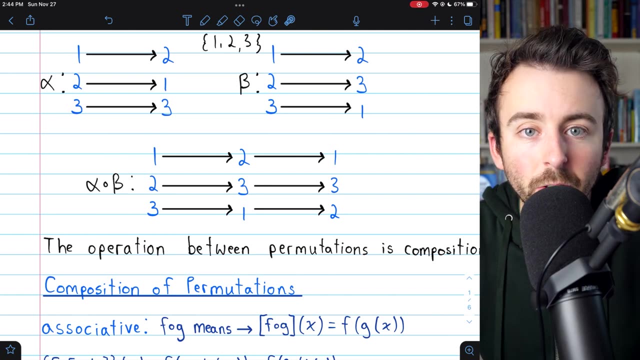 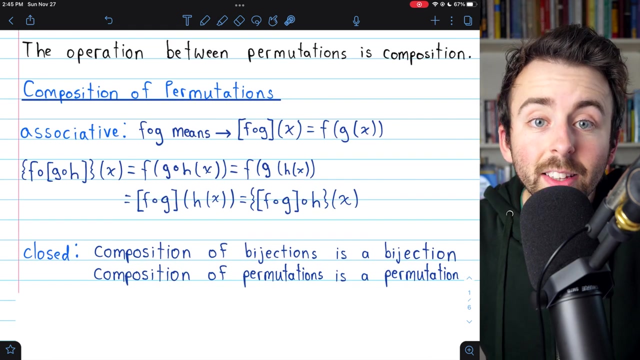 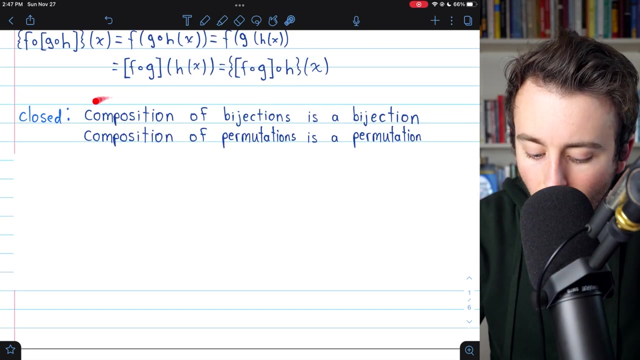 g of h of x and so indeed composition between permutations more generally function composition itself is associative earlier we took the composition of two permutations and got another permutation this is of course true in general that the composition of permutations is closed this is because if we compose bijections from a set a to itself we will get another bijection from the set a to itself so if we just have a bunch of permutations of the set a and we compose any two of them we'll just get another permutation on the set a i'll leave a link in the description to my lesson proving that the composition of bijections is a bijection which thus gives us this result of closure for permutations but i hope you'll agree it's a fairly easy result 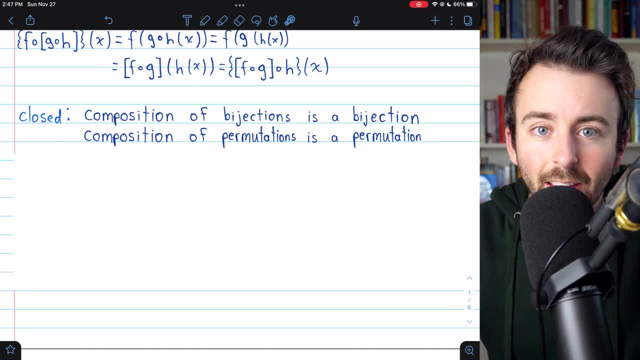 to accept each permutation just shuffles a set into some order and so if we permute a set and then permute it again which is composing permutations you're just going to get the set shuffled in some order so again you're going to get a permutation on that same set moving on 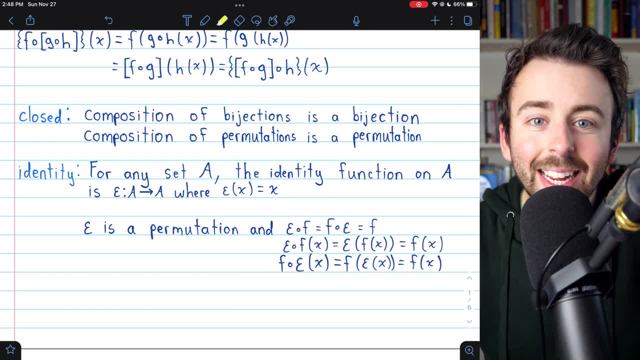 let's quickly talk about the identity do we have an identity element when it comes to composing permutations we certainly do for any set a the identity function on a basically it's a set of masterdam's pseudo polygons which we set in a set of borders which is the identity function on falls intoknown as the identity function on a is this guy we could call epsilon. It goes from a back to a, and it takes each input and leaves it unchanged. So the identity function epsilon of x equals x. Certainly by definition, this epsilon is a permutation. It is a bijection from a to itself. And we see if we compose epsilon with any other permutation, that just gives us the permutation right back. This is fairly easily demonstrated as I wrote out in these equations, just explaining this one, for example. If we compose epsilon with any permutation f, by definition, that's taking f and plugging it into epsilon. But epsilon doesn't change the input, so we just get f back out. So epsilon of f is f. So indeed, epsilon is our identity element. 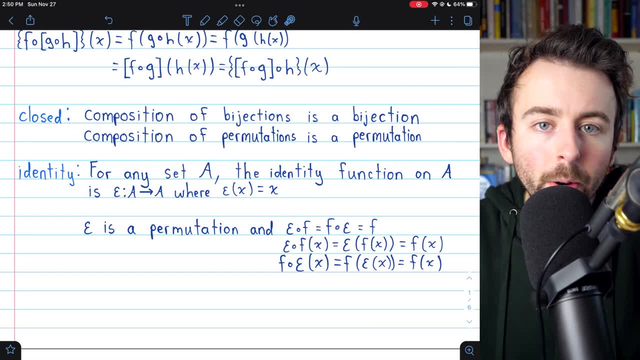 When it comes to composing permutations, if we compose any permutation with this identity 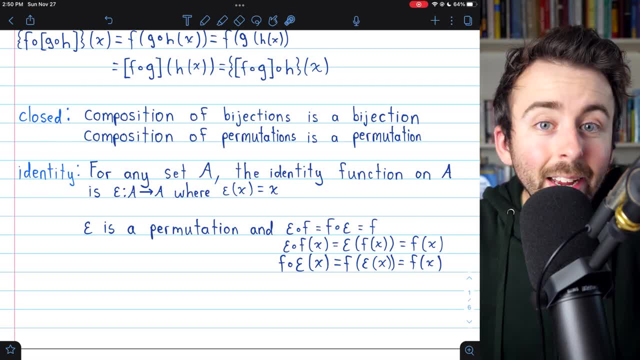 function, the permutation is left unchanged. Now that we have an identity element, we can start 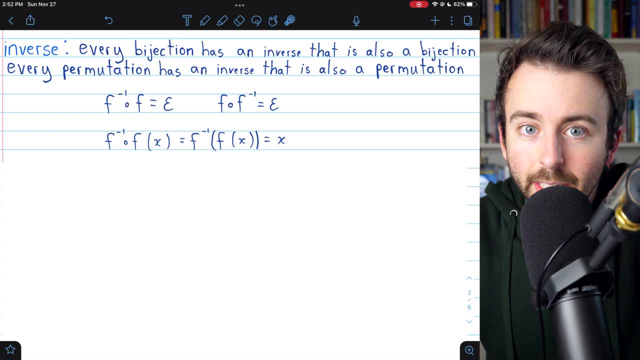 to think about inverses. Recall that permutations are just bijections from a set to itself. Hopefully you're familiar with the fact that bijections have inverses, and I'll leave a link in the description to my lesson proving it if you need to see that. But we know everybody bijection has an inverse that is also a bijection, and thus every permutation has an inverse that is also a permutation. Now we need to be careful. We're talking specifically about inverse functions. This doesn't necessarily mean that these inverse functions are the inverses in the context of the groups that we're trying to create, but we can quickly check that in fact they are exactly what we're looking for. If we have an inverse function, f inverse, composed with the original function f, by definition we get the identity function. 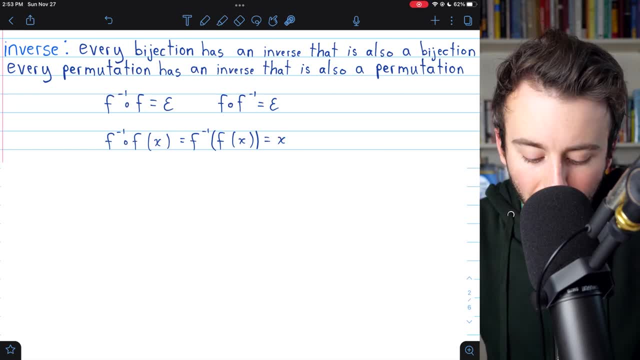 And here's some of the details of that written out in one direction. If we take f inverse, which could just be the inverse of a permutation, and compose it with f itself, well by definition that means we're plugging f of x into f inverse, but by definition of inverse functions, and in this context inverse permutations, we get the identity function. So if we take f inverse, and we 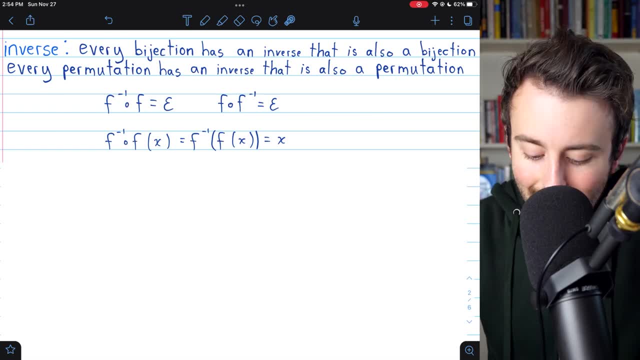 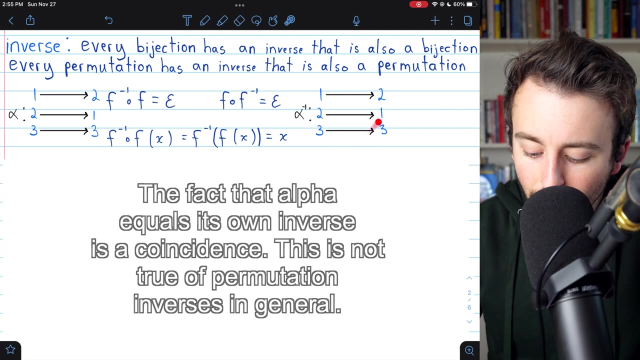 end the permutation, we just undo each other leaving the inside element x unchanged so we have inverse elements for our permutations. Going back to the first permutation alpha that we saw at the beginning of the video, this would be alphainverse, which sends 1 to 2, but alphas inverse element sends 2 back to 1, the inverse of R times 0 to one which is alpha, and the inverse of 1ru, which sends 1 to two gives us 1 sub cha. Now now as we move over here here, if the previous permutation value itself parts in dir, it can't go through the buffer, we're relatively a Hessen perguntk unity, and we say that that point was ¯0 Mensch the Bleue는데, as long as this value is alphainverse mean to ал knappien America. Like alphainverse even though this restriction맛 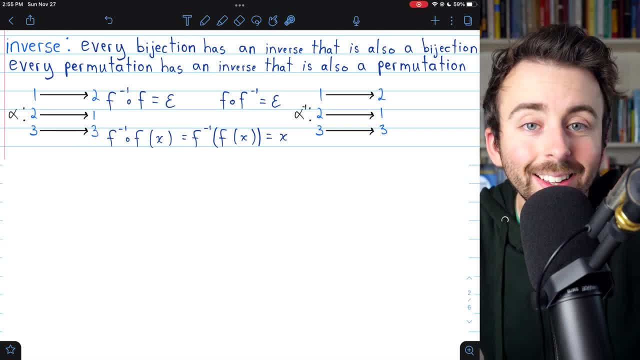 one, but alpha inverse sends one back to two, and they both leave three unchanged. If we permuted a set with alpha and then with alpha inverse, the set would be unchanged. If we permuted it with alpha inverse and then alpha, it would also be unchanged. If you compose a permutation with its 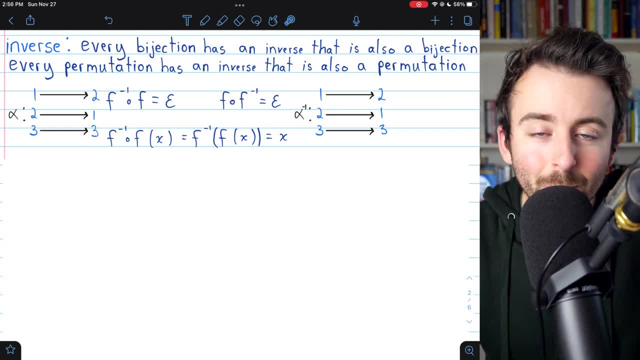 inverse, that ends up not changing anything at all. You get the identity. So we've got inverse elements, we've got an identity element, we've got closure, we've got associativity, we've got 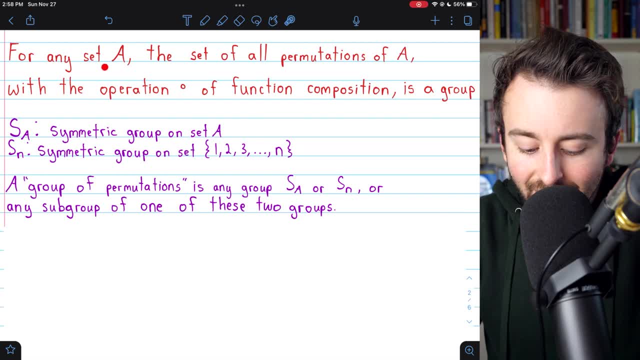 groups. And that's our big result. For any set A, the set of all permutations of A, the set of all 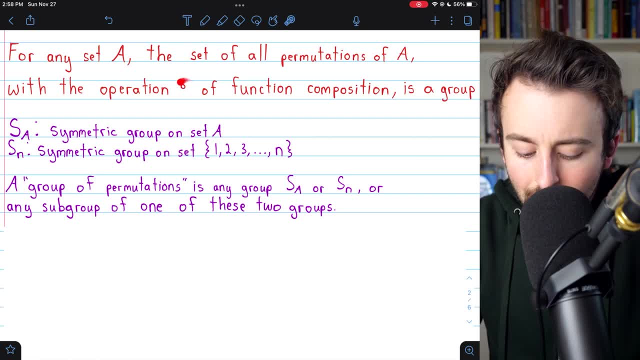 bijections from A to itself, along with the operation of function composition, is a group. These are groups of permutations. Here's some common notation. S sub A stands for the symmetric group on the set A. 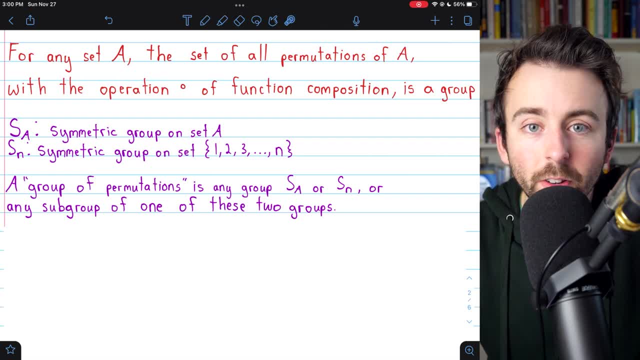 This is just the set of all permutations of A. It's called a symmetric group because each permutation of a set is like one of the set's symmetries, very much like how you could rotate a square and place the square back onto itself. You can permute the elements of a set and place 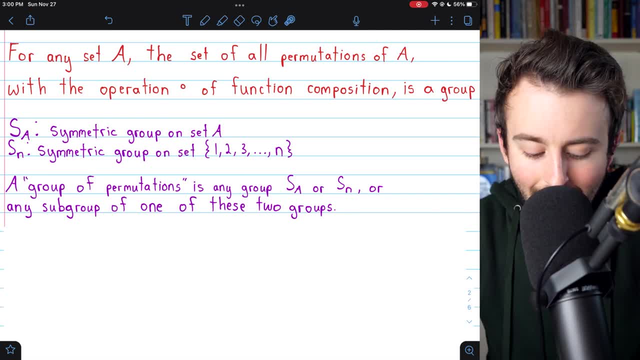 them back onto the set. That's like a bijection, right? And then S sub N, this is the symmetric group specifically on the set of the set A. 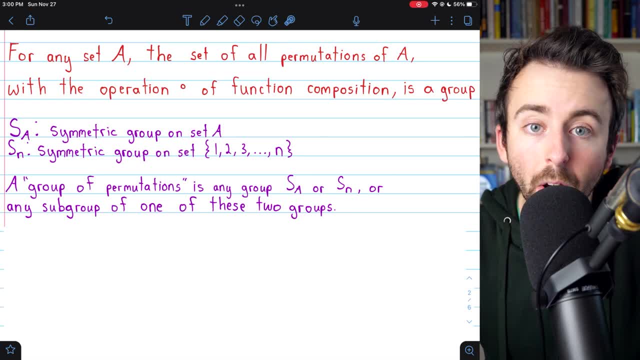 The first N positive integers. So the group of all permutations of 1 through N. And then generally, if we say a group of permutations, we're referring to any group S A or S N, any of these symmetric groups, or any subgroup of one of these two groups. So a symmetric group S A has all permutations on the set A, but a group of permutations doesn't necessarily need to have all the permutations. 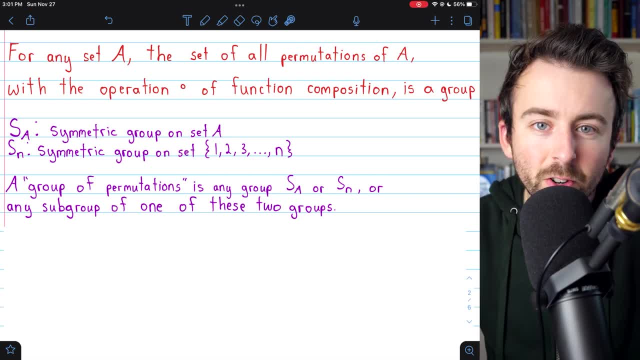 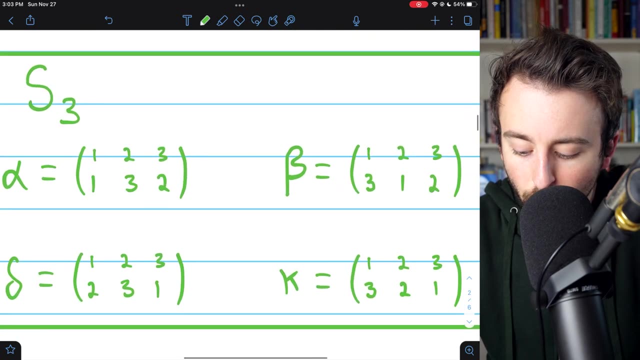 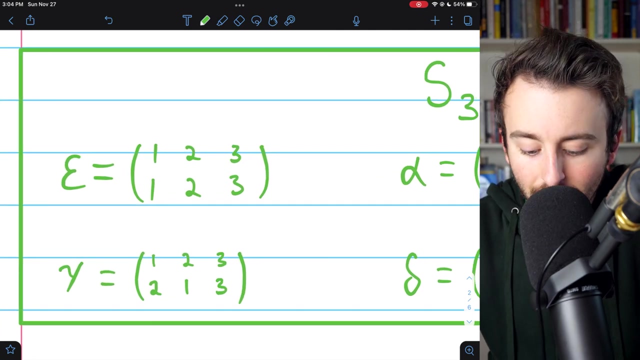 So when we say a group of permutations, we could be referring to a subgroup of a symmetric group. It doesn't necessarily have to be the whole symmetric group. Let's dig more into detail with an example. Here is the full symmetric group S3, every permutation on the set of positive integers 1 through 3. As you might expect, there are six elements. You may recall that the number of permutations on the set of positive integers 1 through 3 is the number of three objects is three factorial. So unsurprisingly, we have six different permutations 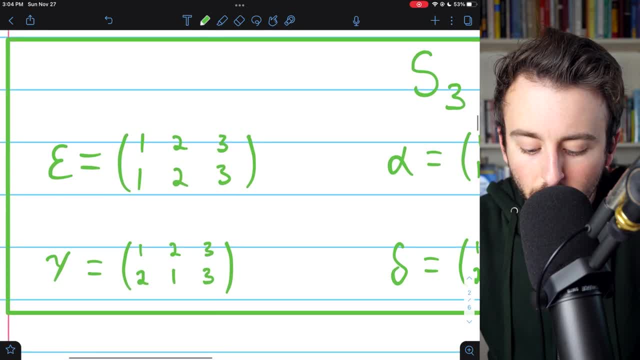 here. The notation I've used is a common notation for permutations that I think you'll agree is pretty straightforward. Here for epsilon, what this notation means is that the permutation epsilon takes 1 and sends it to 1, takes 2, sends it to 2. It takes 3 and sends it to 3. This is, of course, the identity permutation. 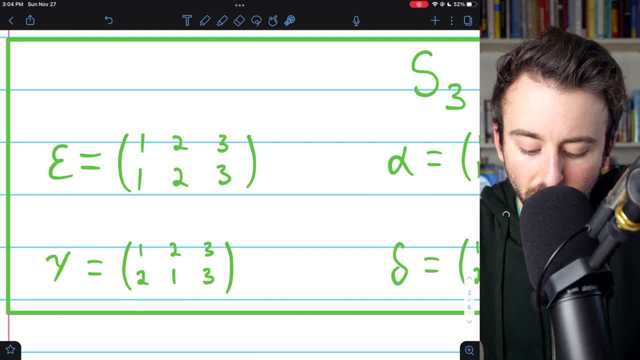 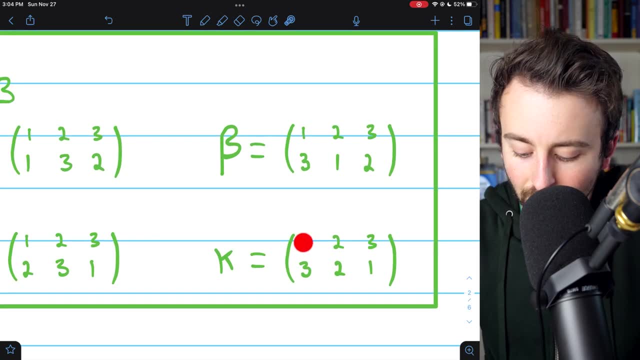 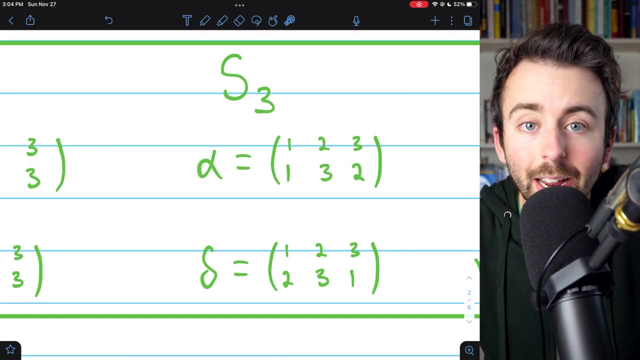 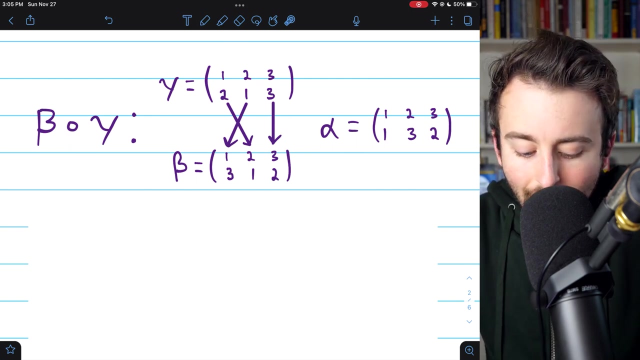 Meanwhile, the permutation gamma sends 1 to 2, 2 to 1, and 3 to 3. If we come over to the permutation kappa, it sends 1 to 3, and so on. So these are all six permutations of 1, 2, and 3. We can try taking two permutations from this symmetric group S3 and composing them. Let's look at beta composed with gamma. Remember, when doing function composition, the function on the right acts first. So first, we would apply this permutation gamma. It sends 1 to 2, 2 to 1, and 3 to 3. Then we apply beta. Beta sends 2 to 1, it sends 1 to 3, and it sends 3 to 2. So the net effect of this composition is that 1 gets sent to, let me make my highlighter, 1 gets sent to 1 because gamma sent it to 2, but beta sent 2 back to 1. 2 gets sent to 3 because gamma sends 2 to 1, but beta sent 1 to 3. And 3 gets sent to 2 because gamma sends 3 to 3, but beta takes 3 and sends it to 2. If you look back at the list of permutations of S3, it turns out that when we compose beta with gamma, what we get is alpha. Our composition sent 1 to 1, just like alpha does. It sent 2 to 3, just like alpha. And it sent 3 to 2, which is also what alpha does. This, of course, isn't a surprise that composing the permutations would give us 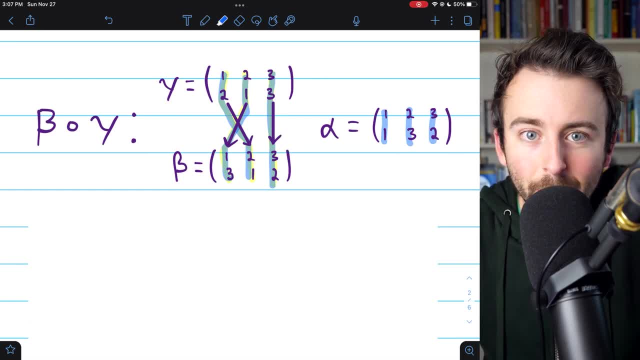 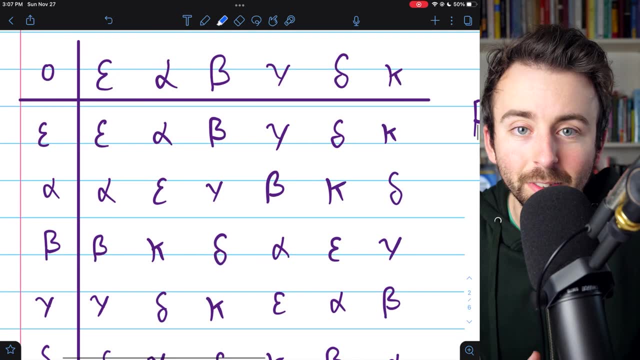 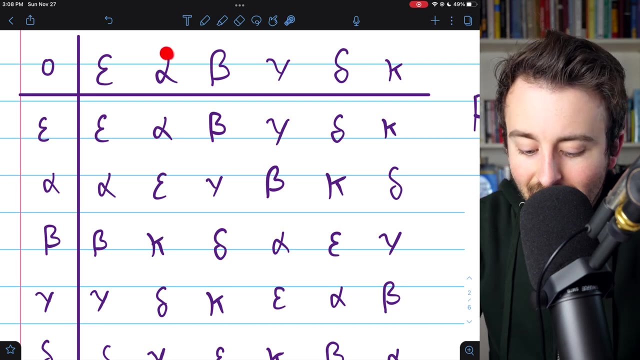 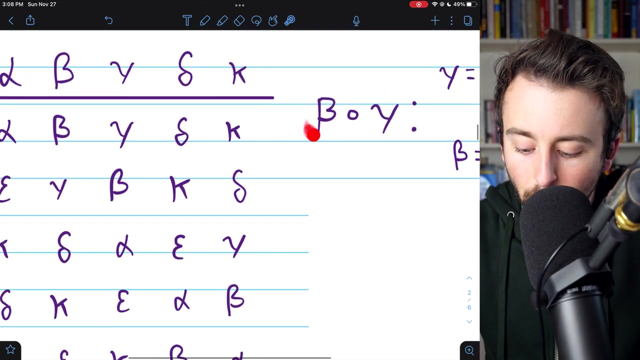 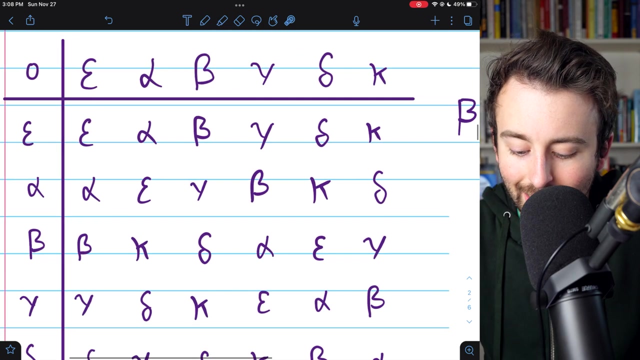 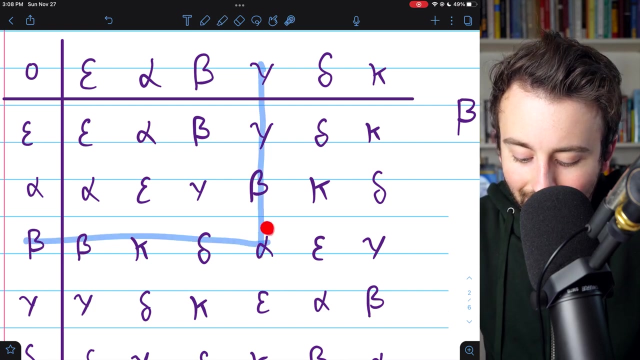 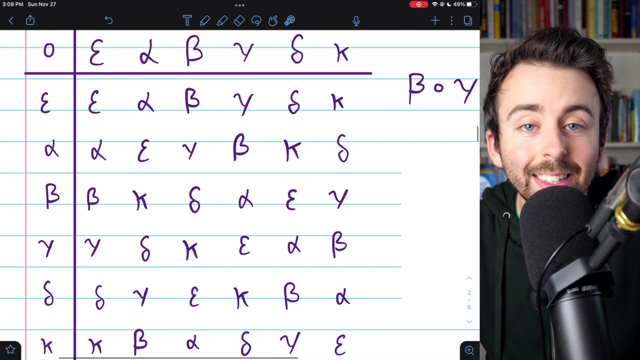 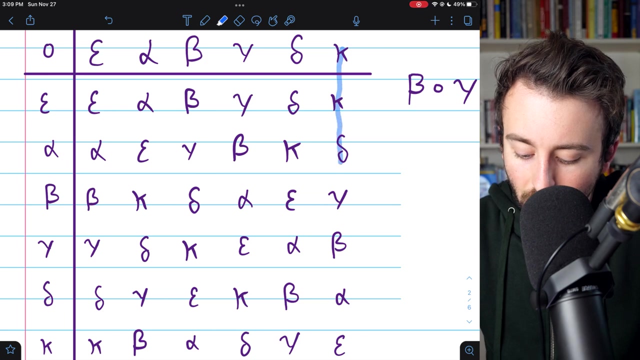 another permutation. Let's now take a look at the full table. If we compose any two permutations from S3, what permutation do we get? Here's the full results. In this table, the function that would act first, the one that would be on the right if you did function composition, is in the top row. And the function that would act second, the function that would be on the left in function composition, is here on the leftmost column. So if we want to look, for example, at what we get if we compose beta with gamma, we would go to gamma first, the function on the right. So look at gamma in the column, and then go down to the beta row. And what we get, no surprise, is alpha. And this is the full table showing us what we would get if we composed any two of these permutations together. If we looked at gamma of kappa, for example, we would start at kappa and go down to the gamma row. That turns out to be beta. 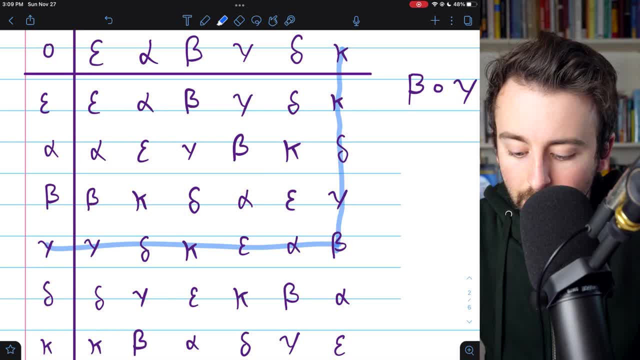 If we want to see what beta is, we would go down to the gamma row, and then go down to the gamma row. beta of alpha would be. We'd start at the alpha column, and go down to the beta row. We see that 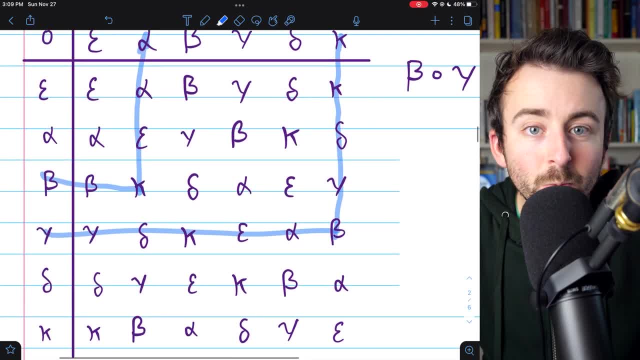 that gives us kappa. These are the full results. Feel free to check them yourself as a fun exercise. 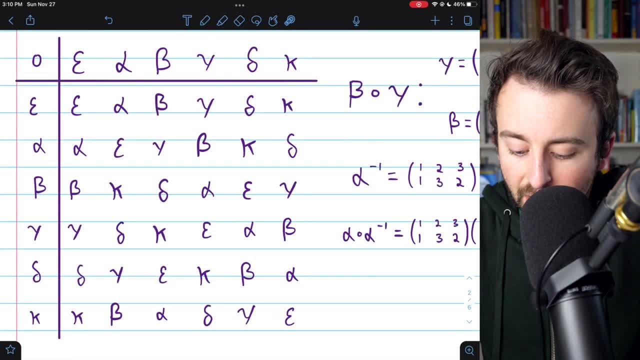 Using this table, we can also pick out inverse permutations. If we look at delta, for example, we see that we get epsilon, the identity function, when delta is composed with beta. So delta and beta are inverses. If we go to the beta, we see that delta is composed with beta. So delta and 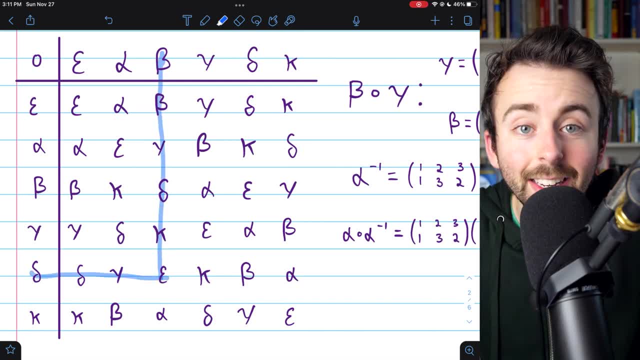 beta are inverses. If we go to the beta column, we get the identity function at the delta row. 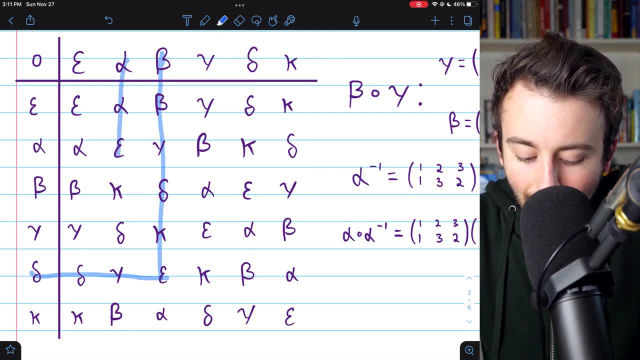 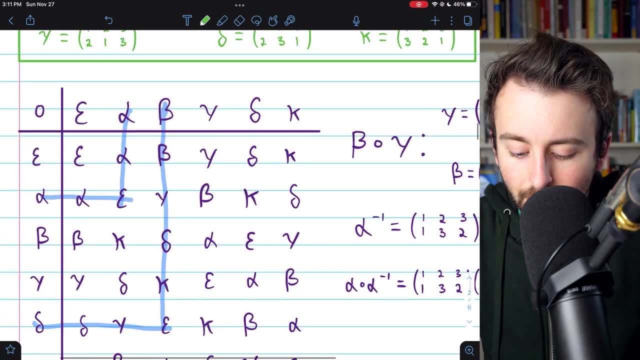 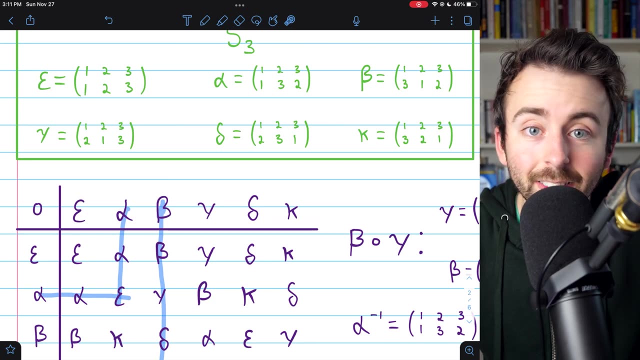 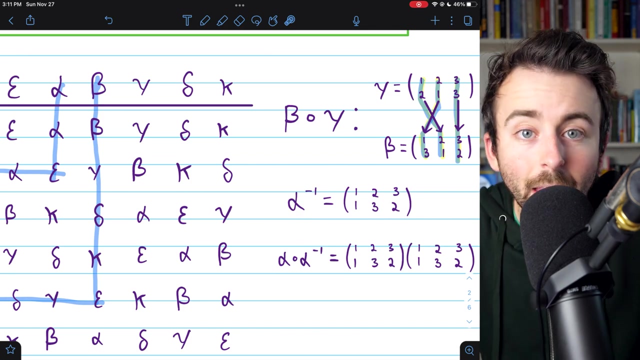 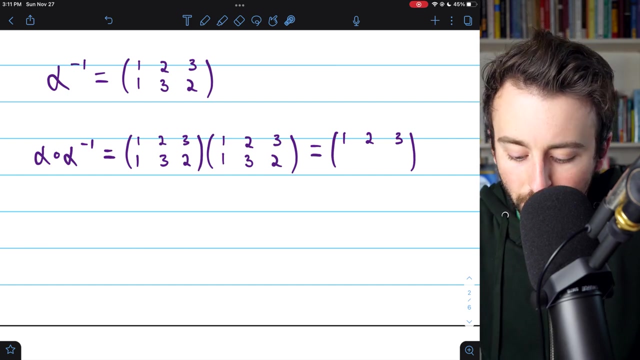 The inverse of alpha, interestingly, is alpha. Alpha is its own inverse. Let's quickly go through that calculation. Alpha is the permutation that sends 1 to 1, 2 to 3, and 3 to 2. Its inverse, based on the table, is itself. So let's try taking alpha inverse and composing it with alpha, and see what we get. When composing permutations, another way we can write them is like this, in this sort of product notation. And again, it's function composition, so we want to go from right to left, starting with this permutation, and then going to that one. So let's look at where 1 would get sent. Alpha inverse sends 1 to 1, and then alpha sends 1 to 1. So 1 just goes to 1. 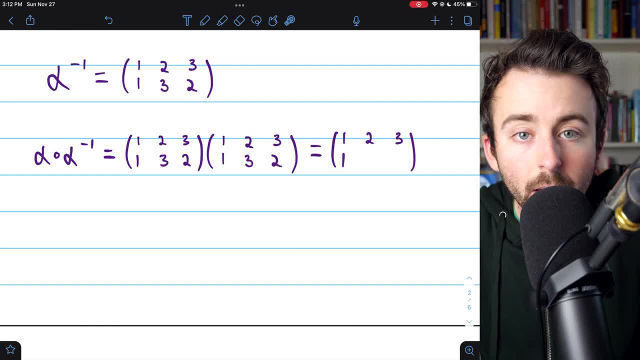 Alpha inverse sends 2 to 1, and then alpha sends 1 to 1. So 1 just goes to 1. Alpha inverse sends 2 to 3, but then alpha sends 3 back to 2. So if we put 2 in this composition, it will first get sent to 3, but then get sent back to 2. And then 3 gets sent to 2 by alpha inverse, and then alpha sends 2 back to 3. So no surprise, if we compose alpha with its inverse, which happens to be itself, 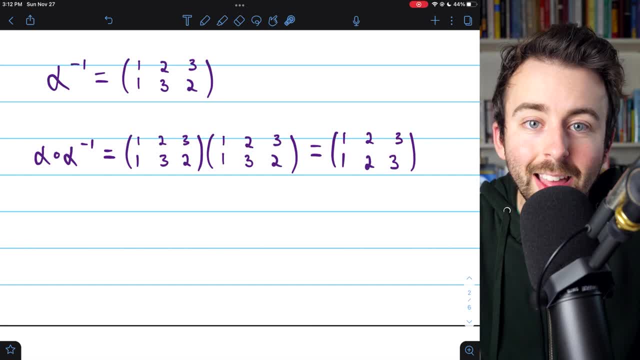 1 just gets sent to 1, 2 to 1. 2 to 2 and 3 to 3. There is just an identity permutation of nothing being moved at all. 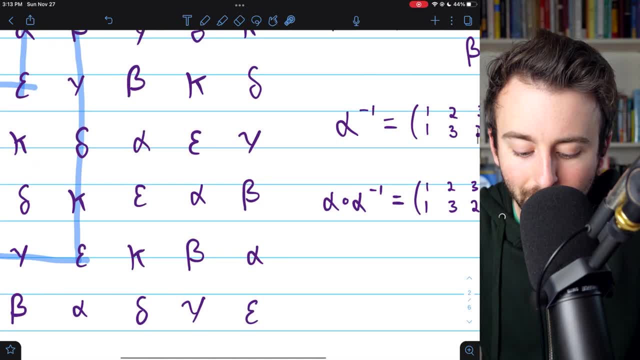 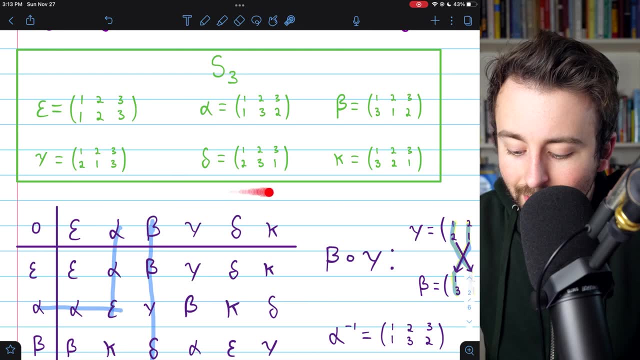 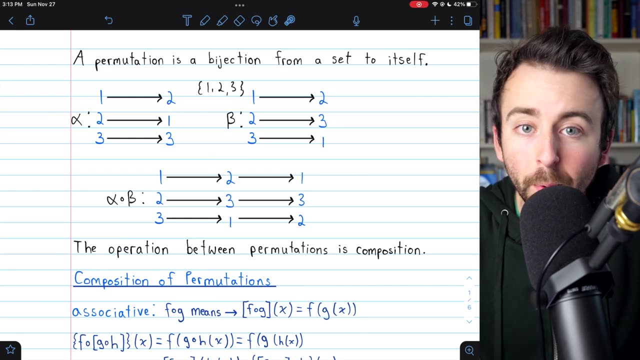 This is, of course, what you'll get if you take any permutation from this table and try composing it with its inverse. And if you want to try doing a few more of those on your own, here again is the complete list of the six permutations of S3. And I think that's enough for now. Remember, a permutation is just a bijection from a set to itself. We can combine permutations,